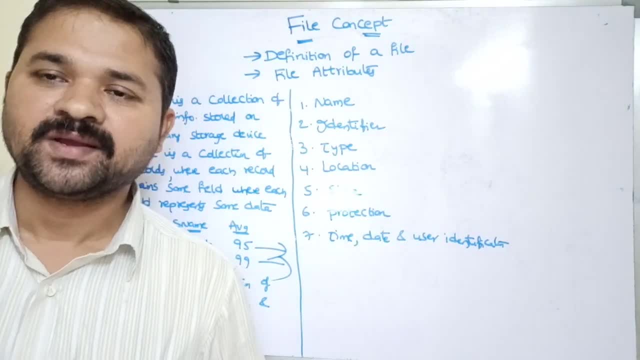 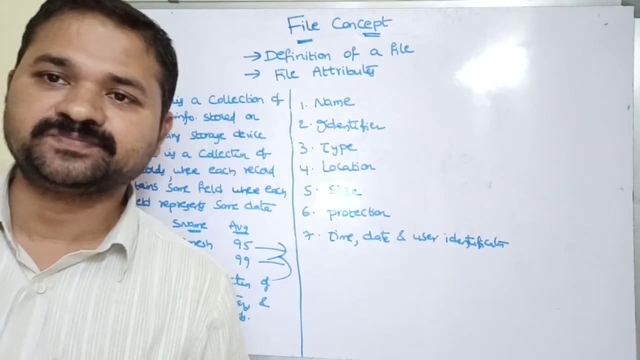 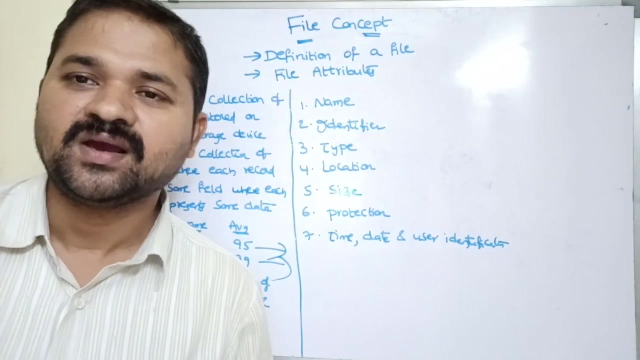 alphabets, digits and symbols. A file can be a source file or object file or an executable file. We know what is a source file: It may be some text file or some document file or some ppt file. or, if you take a C language, then it may be a C file or CPP file or Java. 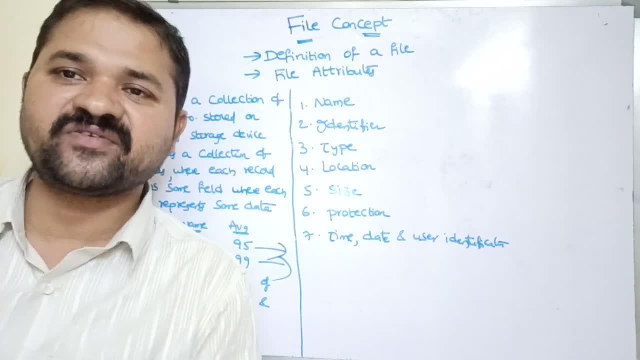 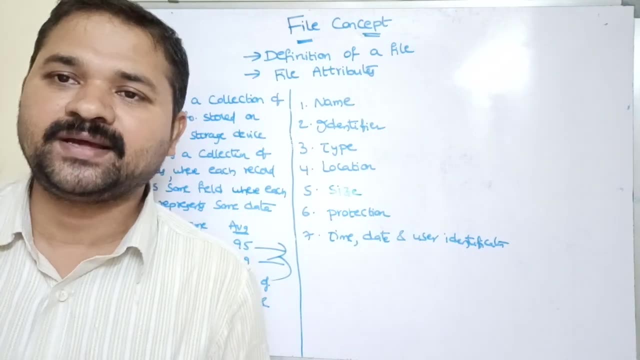 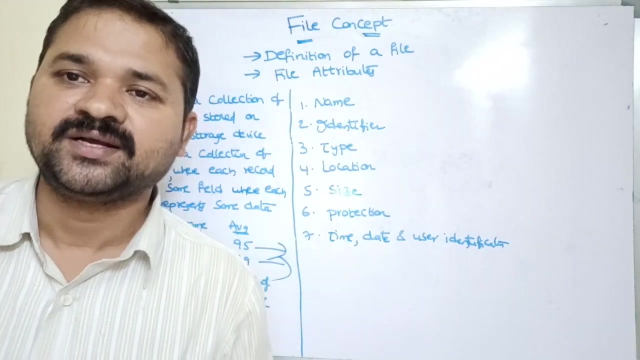 file C, sharp file. So likewise we can have several types of source files, and a file may be an object file. So whenever a file is compiled, then it produces an object file. Object file means the corresponding file is in byte format, that is, in the terms of zeros. 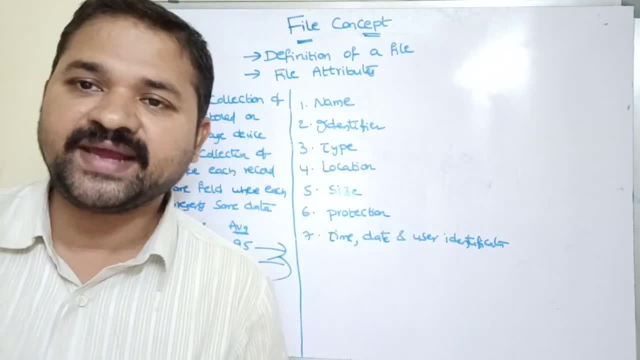 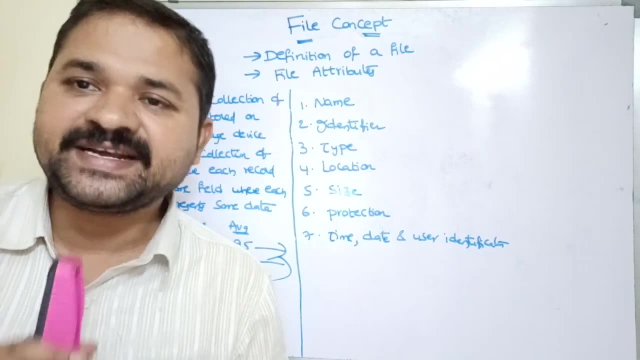 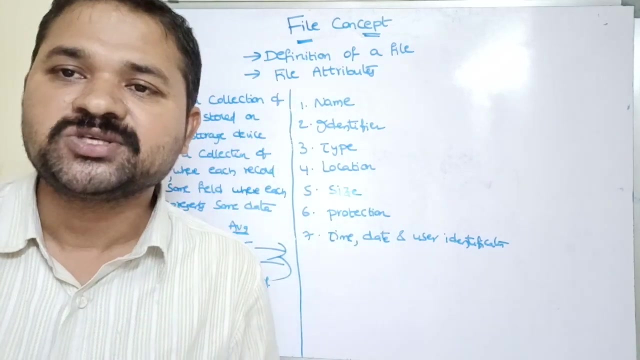 and ones Next. a file may be executable file. Linker produces executable file. So whenever an executable file is created, then it specifies that the file is ready for execution. So the loader loads that file into main memory So that the corresponding file will be executed. So these are the different files here. Now 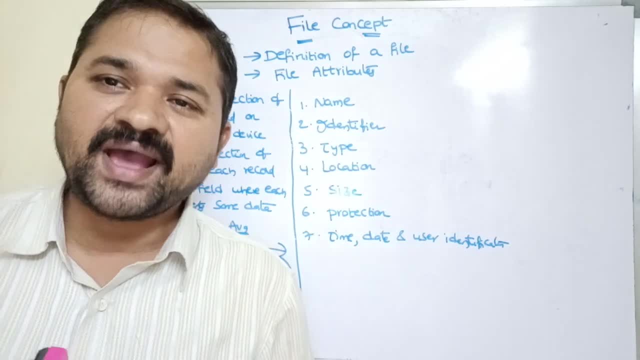 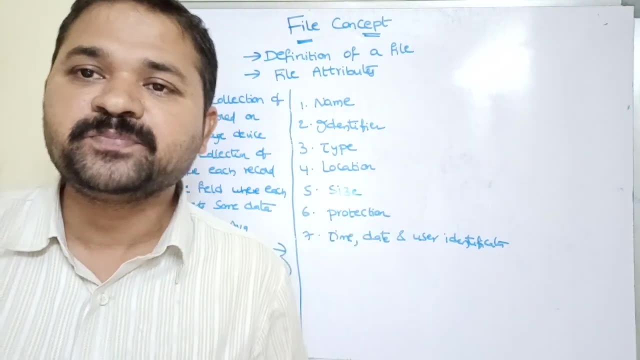 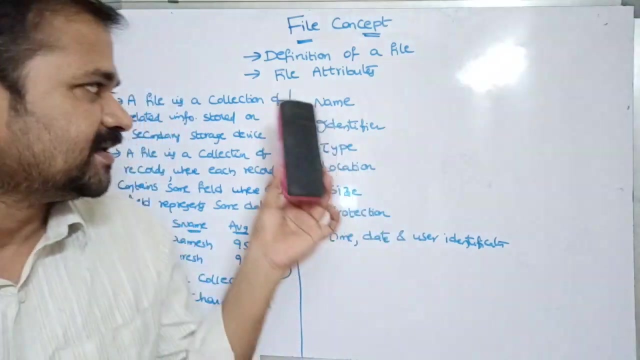 let us see about file attributes. Every file is associated with some attributes. So whenever we save a file, then in addition to the file name, all these attributes will be saved in the hard disk. Here we can have several types of attributes, like name, identifier, type. 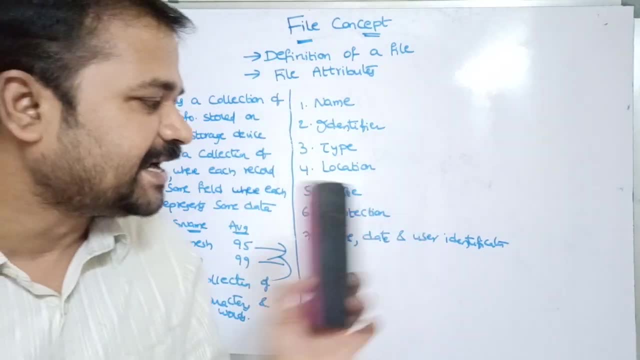 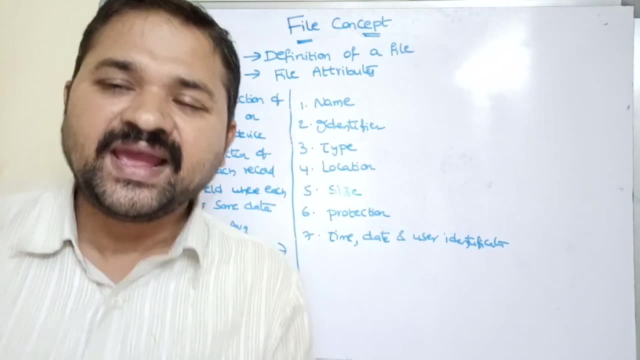 location, size, protection, time, date and year. So these are the different files here: User identification. So let us see all these attributes one by one. So the first one is name. Every file has a name. In order to perform operations on the file, we use a name. Second, 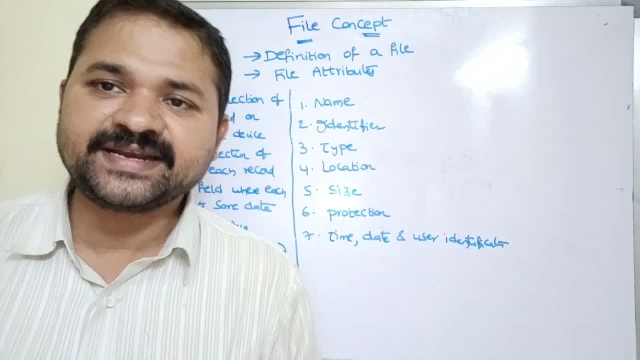 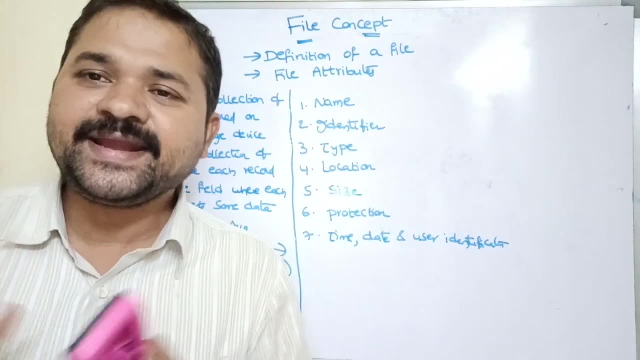